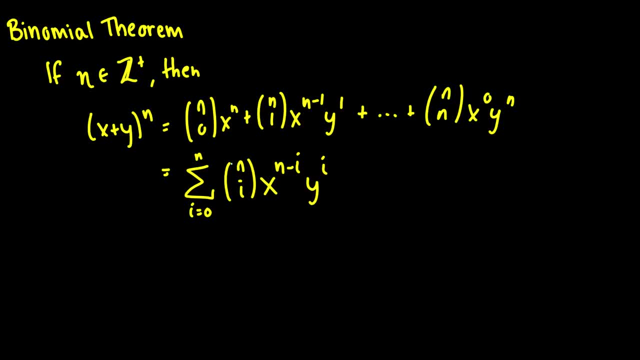 0 times x to the n plus n. choose 1 times x to the n. minus 1 times y. 1 plus dot, dot, dot all the way up to n. choose n of x to the 0 times y to the n. Now we have. 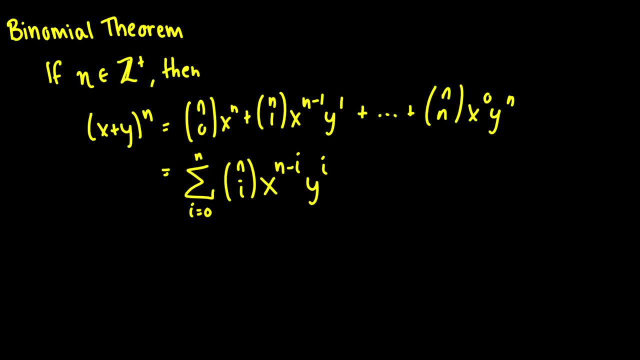 this really convenient notation for this and this is the summation notation. So we have this really convenient notation for this and this is the summation notation That basically you put i equals 0 into the first case and you solve for that. So 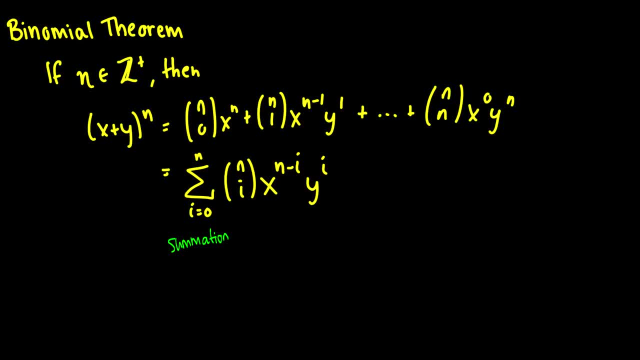 in the first example, if we have i equals 0, we get n choose 0 times x to the n, minus 0 times y to the 0, and then we add the next value of i, so then we add 1 to i, so i is now 1, and we go n choose 1 times x to the n minus 1 times. 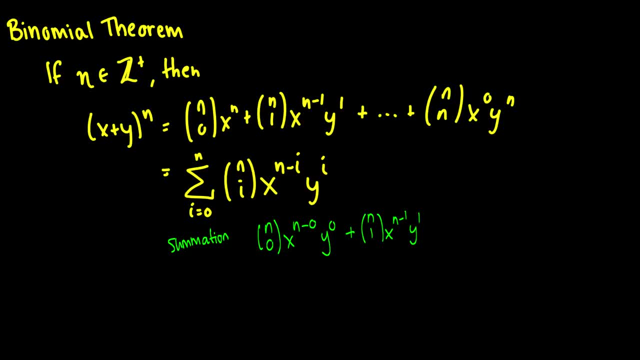 y to the 1, and then we keep going until i reaches n, and you'll see that this is exactly what I wrote up here, just expand it out. So this is a very convenient summation notation. Basically, you start with the largest power of n and then 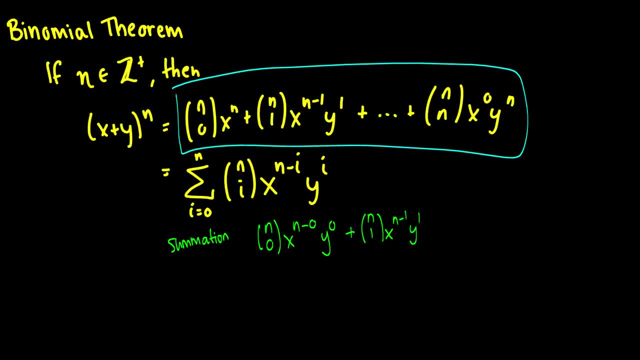 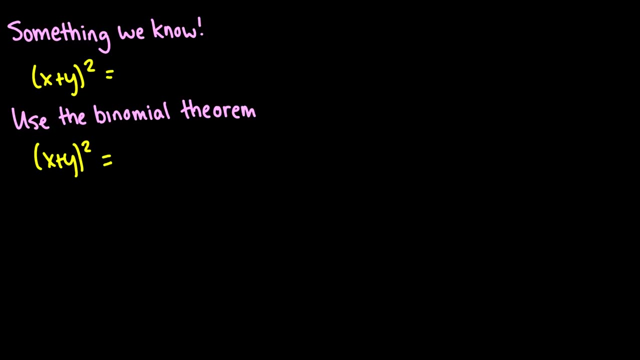 each subsequent addition, you just move one power of x to the n, over to the y, until y then reaches y to the power of n, in a nice informal manner of explaining what's going on here. So let's put it to use. Let's do it the way. 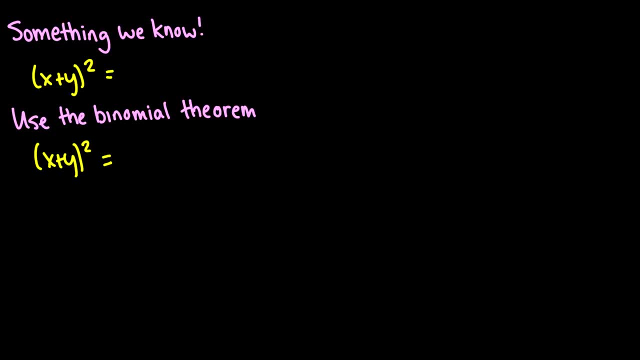 we know, with x plus y raised to the power 2.. Of course we know this is the same thing as x plus y times x plus y, and we can just FOIL this out to be x squared plus x times y plus x, times y plus y squared, which is the same thing. 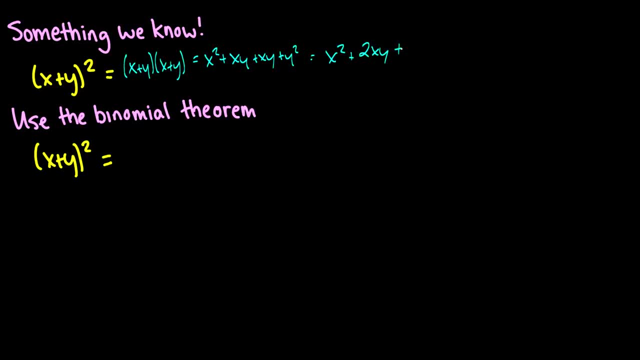 as x squared plus 2xy plus y squared. Now let's do the same thing using the binomial theorem. So first we're going to have 2. choose 0 times x to the 2, y to the 0 plus 2. choose 1 x to the 1, y to the 1 plus 2. choose 2 x to the 0, y squared, so now 2. 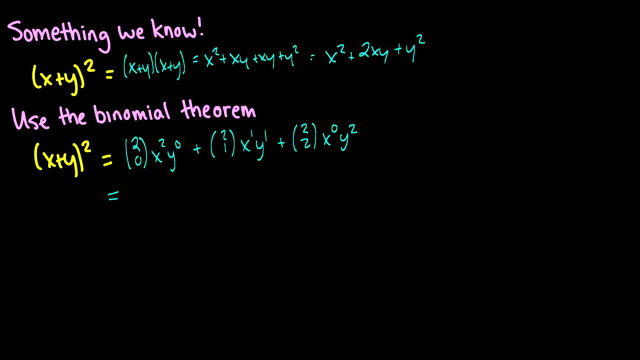 choose 0 x to the 0 y squared, so now 2 chooses 0 x to the 0 x squared, so now 2 is going to be- I'm going to write this on the side: we're going to do all three. 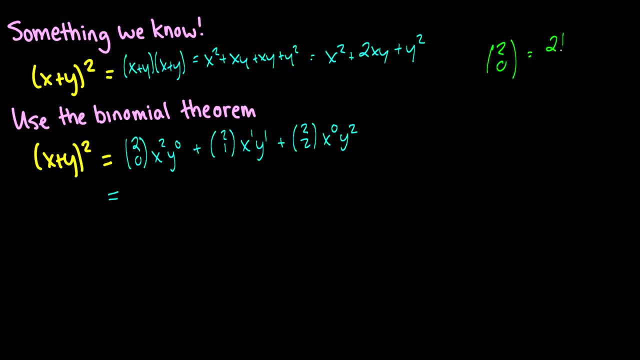 at once: 2 choose 0 is 2 factorial over 0 factorial times 2 factorial, which is just going to be 1.. 2 choose 1 is 2 factorial over 1 factorial times 1 factorial, which is 2, and 2 choose. 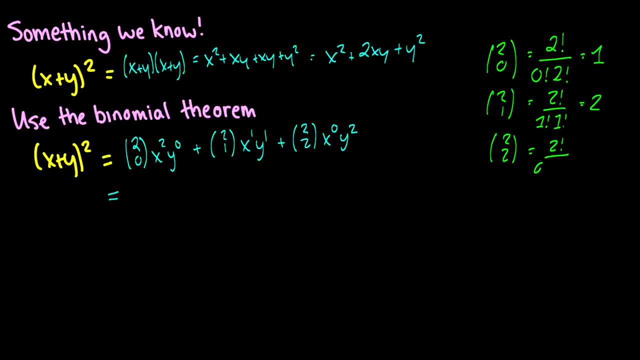 2 is going to be 2 factorial over 0 factorial times 2 factorial, which is 1.. So let's plug those values in. We're going to have 1 times x squared y to the 0 is just 1, so we'll just leave it out. Then we're going to add 2 times xy plus. 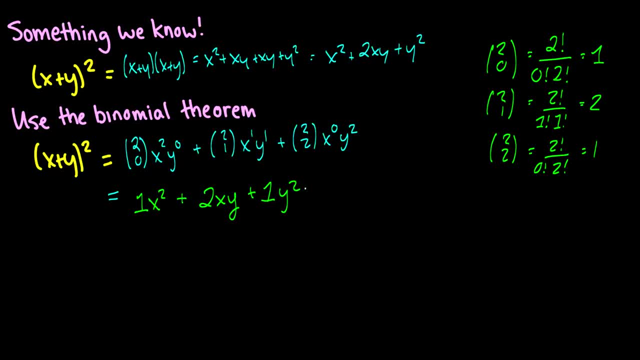 1 times y squared, And in this happens to be the same thing. we got up top, So the formula works for a small power and you can check this for a higher power if you have any questions about that or have any concerns about whether this is true or not. 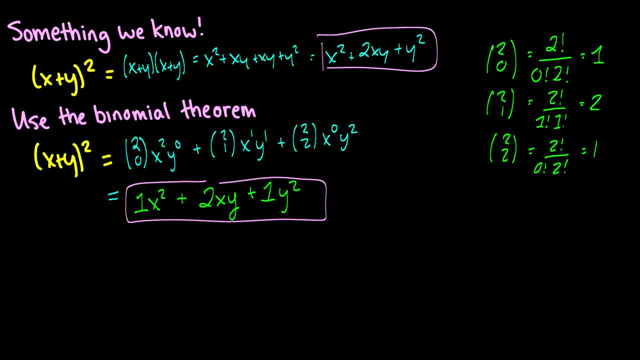 But take my word for it. it is true, And I also want to direct you to another cool thing that we see here, and that is 2 choose 0 and 2 choose 2 have the exact same formula. So here's an interesting thing. I'll write this as a cool. 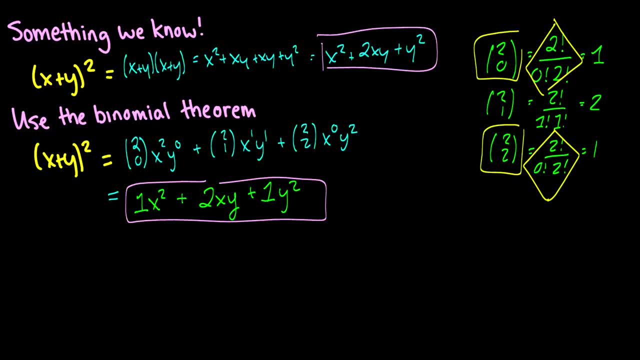 aside for things you can do with combinations: n choose k is the same thing as n choose n minus k, So you can use these interchangeably. As an example, 49 choose 6 is the same thing as 49 choose 43. So there's a cool little thing. 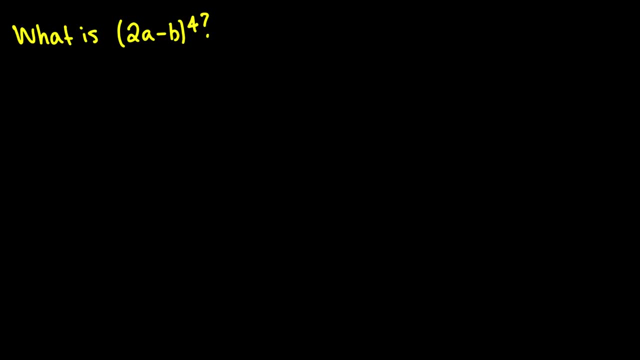 and we're going to see a nice friendly application of this very shortly. But first one more practice problem, And I do this because sometimes when you just say oh, x, y, they both have constant 1 in front of them. so it's not that difficult. But what is 2a? 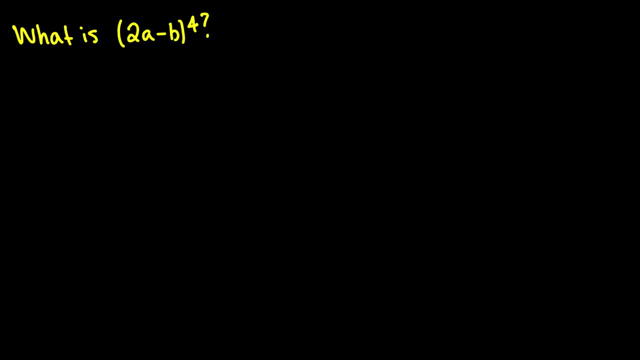 2a minus b raised to the 4.. So I'm going to do this really sort of quick and point out the important things here. So our first one is going to be 4 choose 0.. I'm going to add them all vertically, just easy visually. 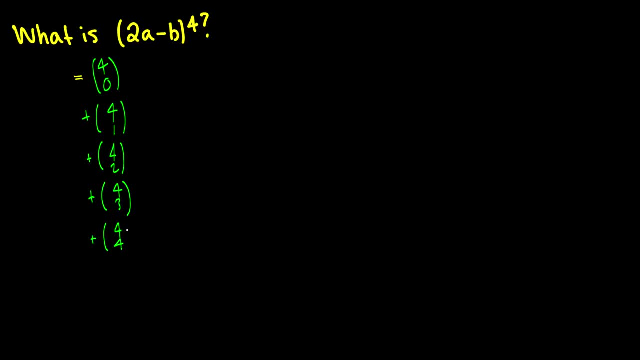 So we're going to have 4 choose 0 all the way up to 4 choose 4.. Our first one is going to be 2a to the 4 times. the first one is going to be 2a to the 4 x 2a to the 4 x, 2a to the 4.. 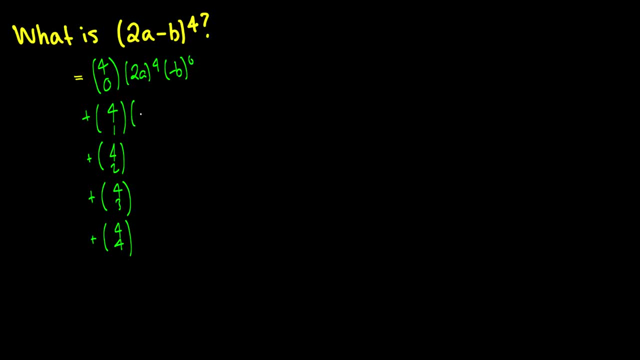 times minus b to the 0, and then we're going to have 2a cubed minus b to the 1, 2a squared minus b squared, 2a to the 1 minus b cubed, and 2a to the 0 minus b to the 4.. I wrote it. 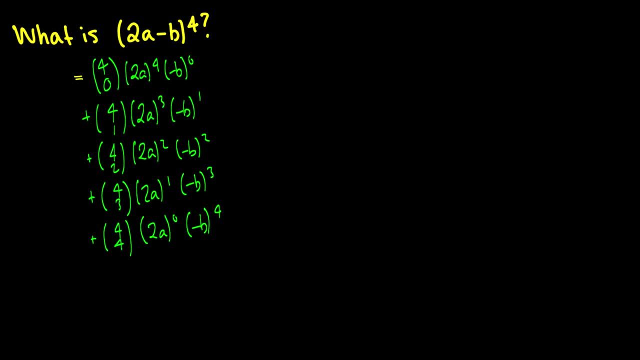 vertically like this, so you could see the progression of step by step what's happening. The power for 2a is decreasing and the power for negative b is increasing. So the interesting thing here to note is that we take this whole 2a and this whole minus b. 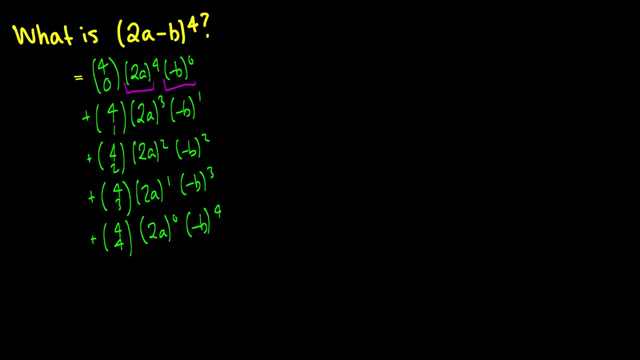 and we stick it into the thing that's getting raised to the power. We basically say x is equal to 2a and y is equal to negative b, and then we plug it into the formula. So the important part here is that you remember. 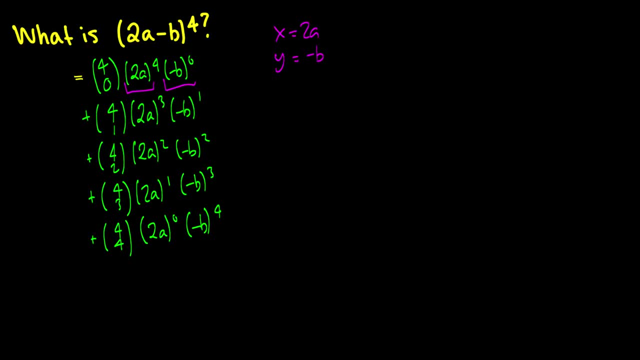 to put the 2 with the thing that's getting raised to the power of 4,, 3, or 2, or 1, because that will change the result if you forget to do that. So we could leave it like this and it would be. 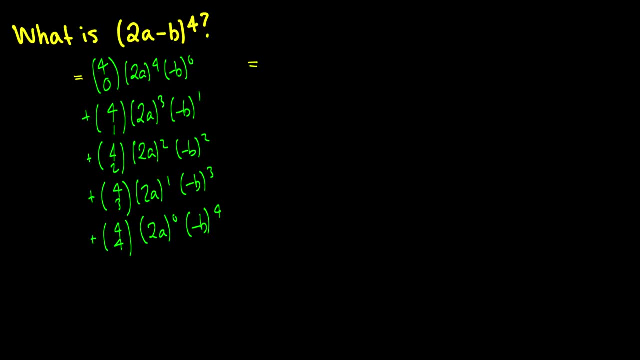 fine. However, I will simplify it a little bit. So 4 to 0 is going to be 1, so we're going to have 1 times 2a to the 4 is going to be 16a to the 4, plus 4 choose 1 is going to be 4 times 8a cubed. but we have negative b. 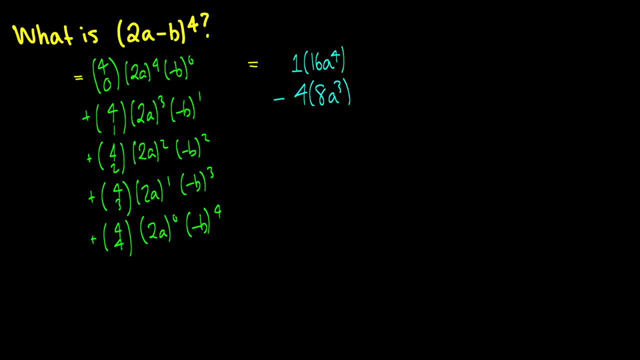 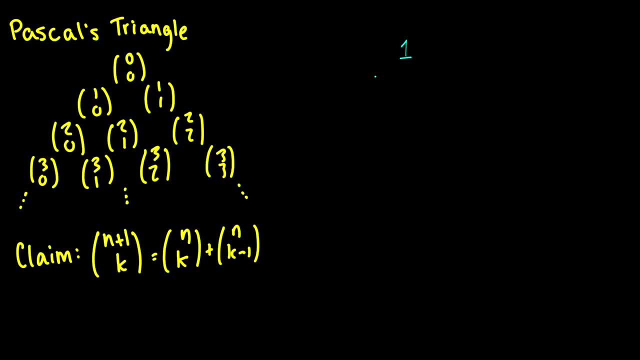 which is going to be 4. factorial over 2: factorial 0 is 1.. Now what is 3? choose 1? Well, if we add the 1 and the 2 together, we get a 3.. So what is 3? 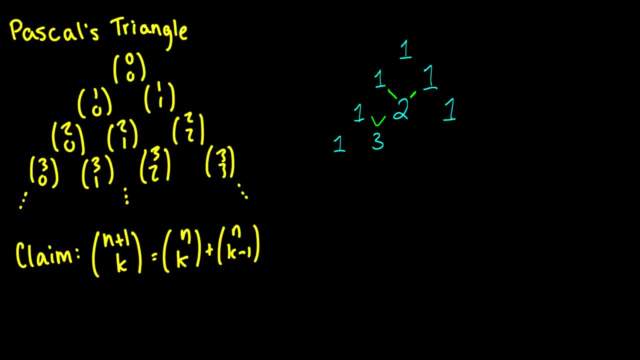 choose 2?? Well, we saw that 3 choose 1 is the same thing as 3 choose 2, which makes sense now because of this cool little Pascal's triangle we have here, And then of course, the outsides will always be 1.. So we have this claim here that n plus 1, choose k is n. choose k plus n, choose k minus 1,. 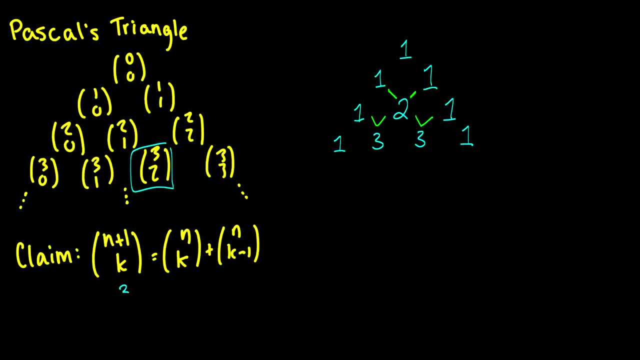 which means, if we take this, 3 choose 2, so we're going to write this as 2 plus 1 choose 2, this should be the same as 2 choose 2 plus 2 choose 1, which we see is actually the same thing. 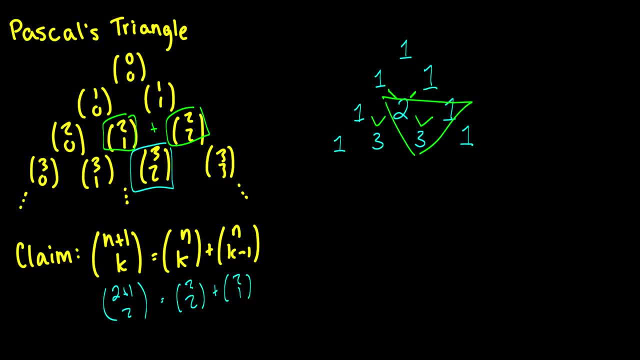 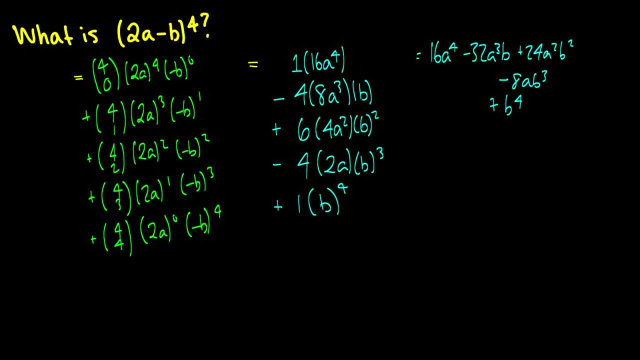 as what we have In this triangle right here. So that's a cool claim, and it turns out that if you break apart the formulas and find an equivalent formula between the two, this holds. So when I went back into this previous problem and I found these numbers right here, you'll notice that after I 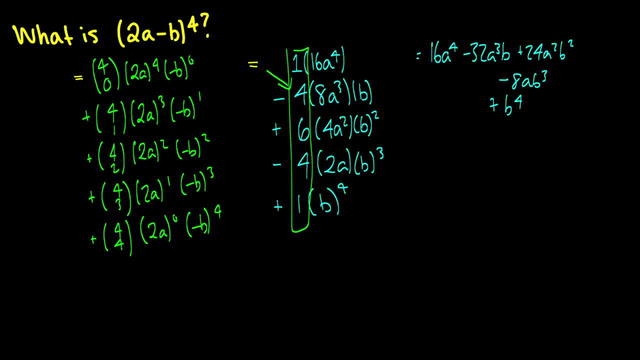 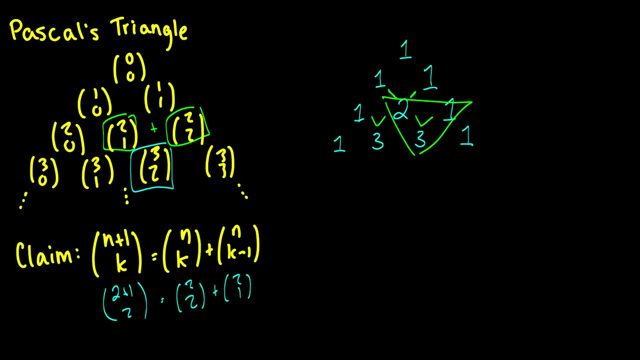 found this 4 right here. it didn't take too long to figure out what the next value was, And that was because you, I was able to figure out the numbers for the triangle at that line, Because if we go next, we know our outers are going to be 1.. Then we have: 1 plus 3 is 4, 3 plus 3 is 6, and 3 plus 1 is 4.. 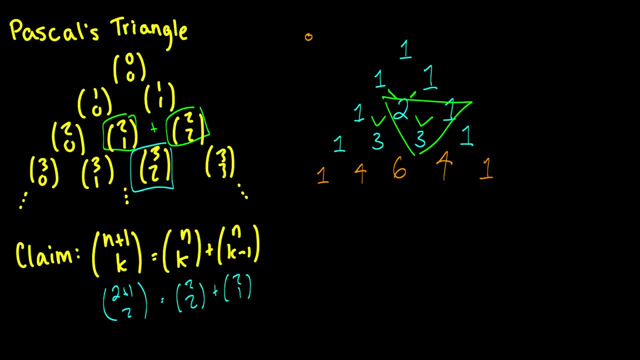 So of course this is x plus y to the 0, to the 1, to the 2, to the 3, to the 4 here. So I want this line, when we deal with something, to the 4, 1, 4, 6,, 4, 1 are the coefficients. 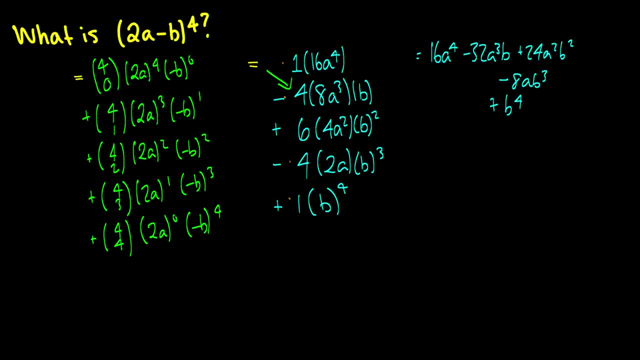 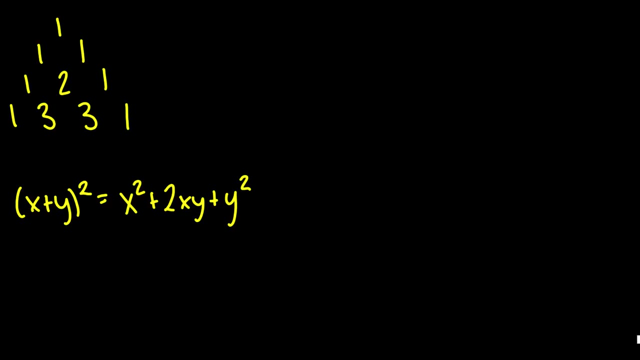 and they just so happen to be 1,, 4,, 6,, 4, 1 here. So that is a very cool trick to help you figure out the coefficients in a much faster manner. So here is another quick example before we go off. 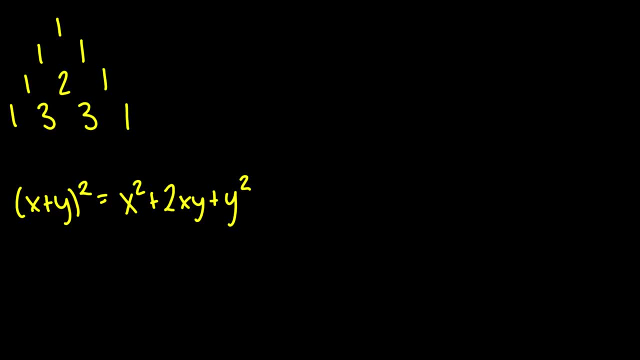 We have x plus y squared is x squared plus 2xy plus y squared, which is very easy to see, is the third line in the table. So what I should say formally is that x plus y to the n takes coefficients of row n plus 1.. 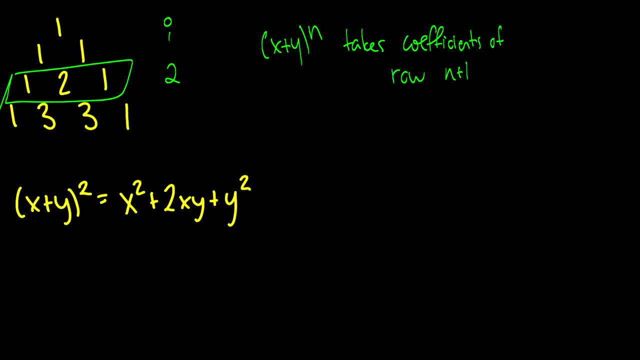 So this is row 0, this is row 1, this is row 2, this is row 1, this is row 2, this is row 3, this is row 4.. So x plus y to the 2 takes row 3.. 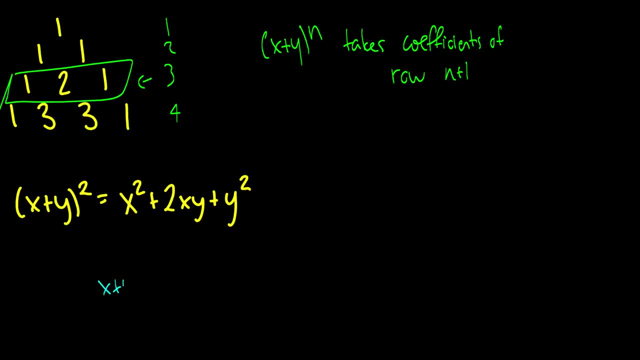 So here is a question: what are the coefficients of x plus y to the 6?? Well, we just draw the triangle so we can actually do this very, very quick. In fact, we have to go up to the seventh line here so we can do that very, very quickly. 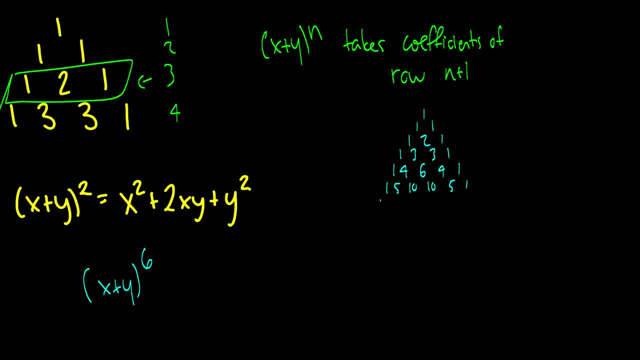 So this is the first, second, third, fourth, fifth, sixth. we just have to go one more line and we will be done. So if we just add up all of the preceding two numbers here, so to get 15,, for example, we took 5 plus 10, to get 20,, we took 10 plus 10 to get 15,, we did 10 plus 5, and this is the coefficients of x plus y to the 6.. 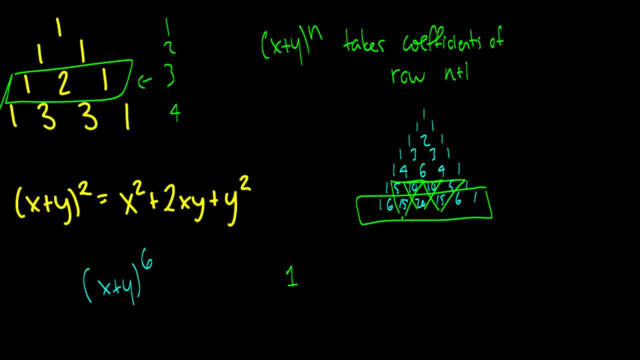 It'll be 1x to the 6.. Plus 6xy to the 5, plus 15,- sorry, x5 times y plus 15x to the 4th, y squared plus 20x cubed y cubed plus 15x squared y to the 4, plus 6xy to the 5, plus y to the 6th. 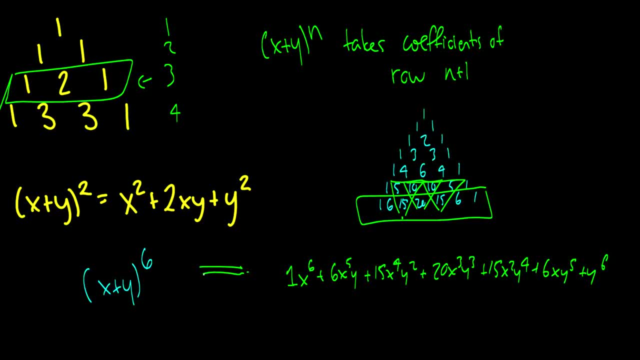 And this is your result, And I could do this that quickly just from Pascal's triangle. So that is really cool. One, you find the row. Two: you remember the pattern for your powers where x starts at the highest and goes down one each addition and y starts at 0 and goes up one each addition until you've filled out that row for the triangle. 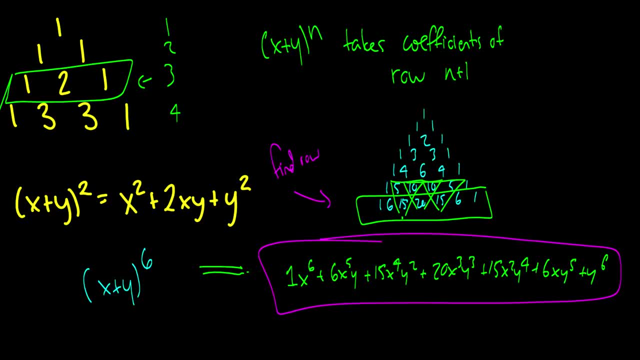 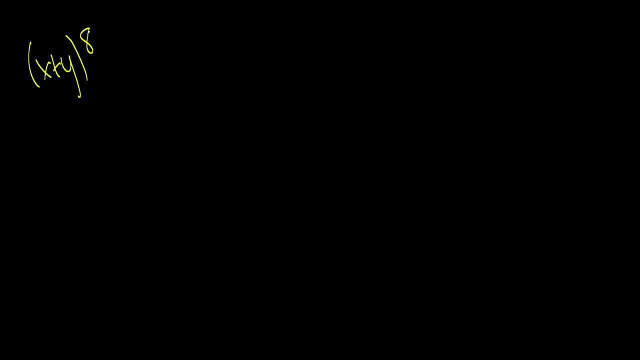 So that is something very cool you can do, And before I go, I am going to ask you to do this on your own: x plus y to the 8, I won't solve it for you, but have a go at it, see if you can do it. 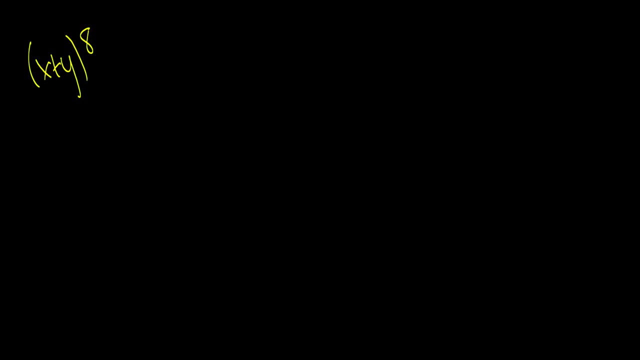 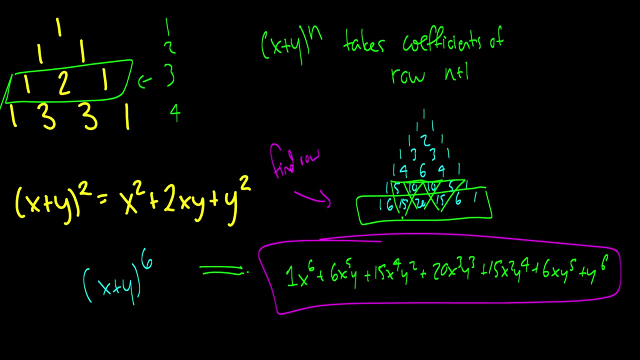 It should be really simple. In fact, if you can remember this, x plus y to the 8, I will even go back to this triangle here- And you just need to extend it two rows, figure out the pattern and see what's going on. 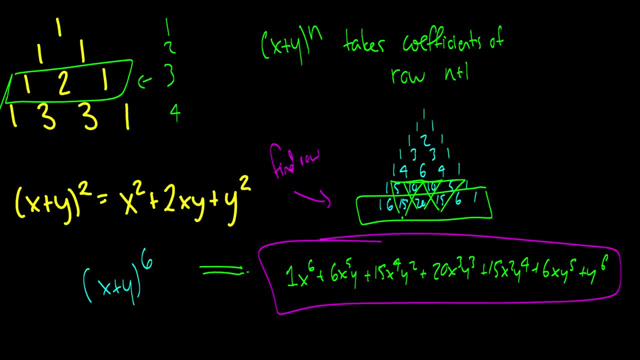 So that was the binomial theorem and Pascal's triangle. If you have any questions on these things, feel free to leave them in the comments and I will get to them As quickly as possible and hopefully clarify any questions you have.